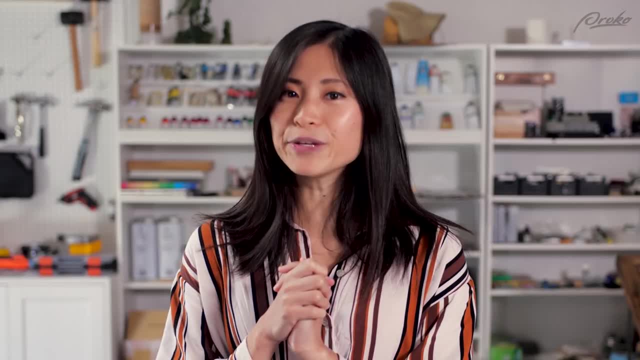 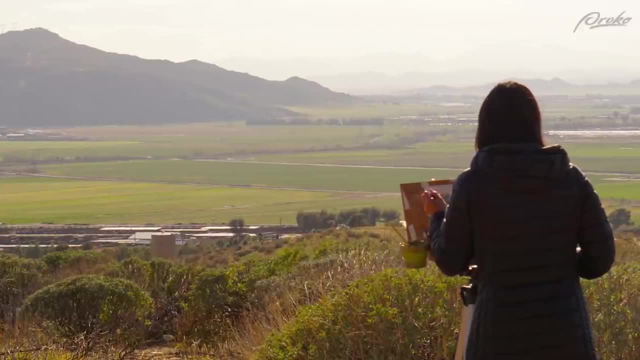 can be so fun at the same time. I have a pretty unique background where I have one foot in the animation industry and another foot in the fine art industry, and working in both mediums has helped me so much in building my own style and my own voice that I can now hopefully share and come. 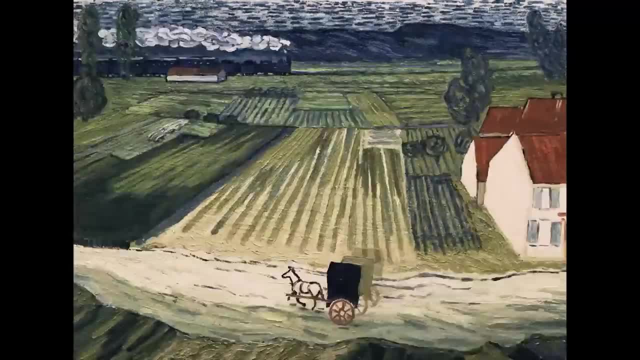 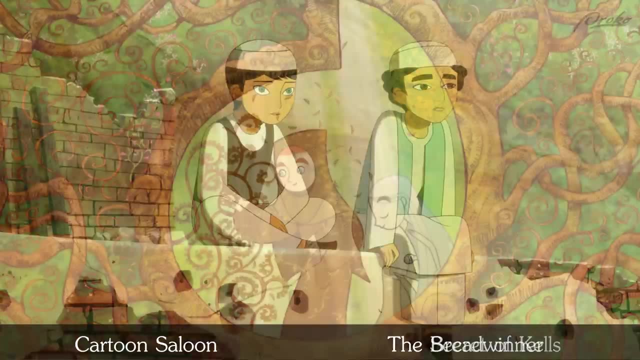 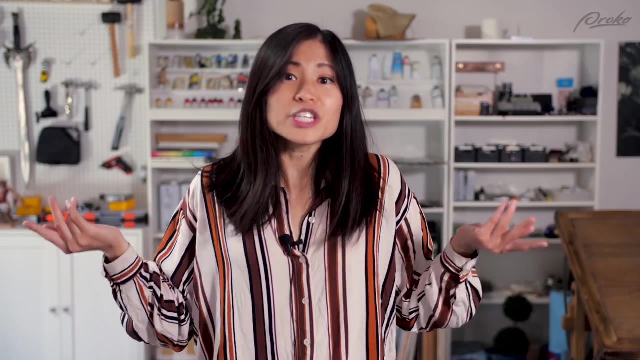 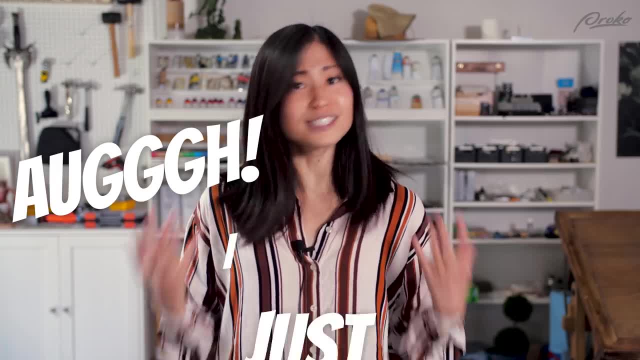 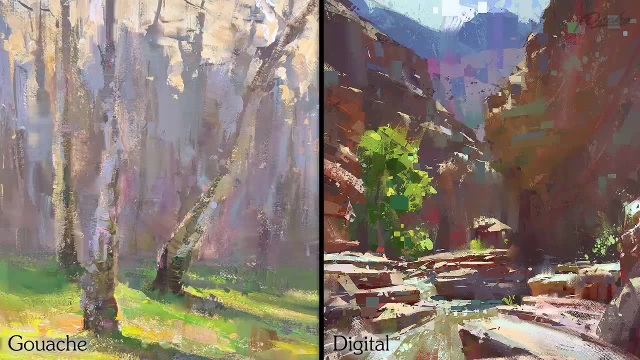 We can't get enough of color. We can't get enough of color. Yet so many times I hear people saying I just can't get the right color. Well, as a gouache and digital artist, painting with gouache has helped me debunk some of the many confusing mysteries that color seems to hold. 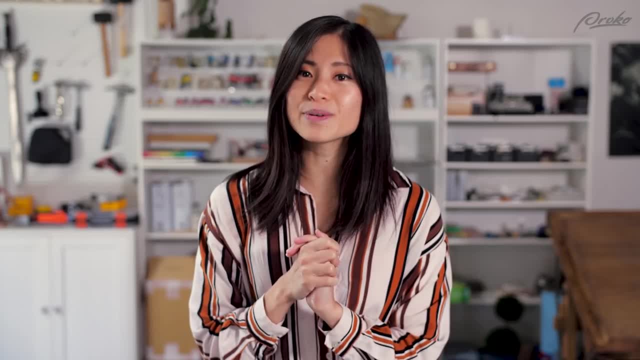 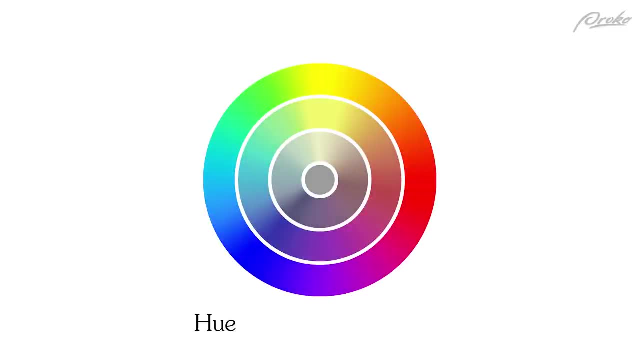 So let's jump right in. First, let's review some basic terms to establish some ground rules. There are three main characteristics of color: hue, saturation and value. Hue simply means the color you are dealing with: Blue is a hue, yellow red is a hue, yellow ochre is a hue. cobalt blue is a hue. 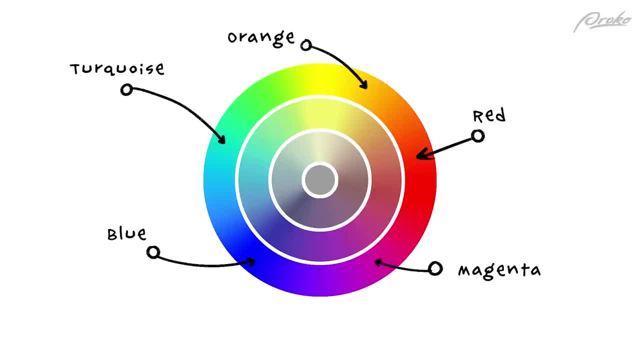 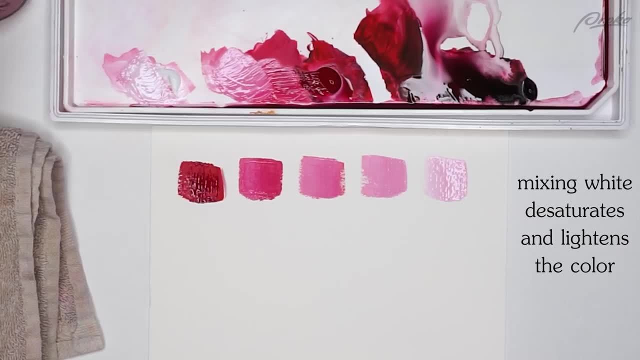 and the list goes on and on until you reach the other end of the rainbow. Saturation is the fancy way of talking about the chroma or color intensity of a color. A fully saturated color is one of pure color and a desaturated version of that color. 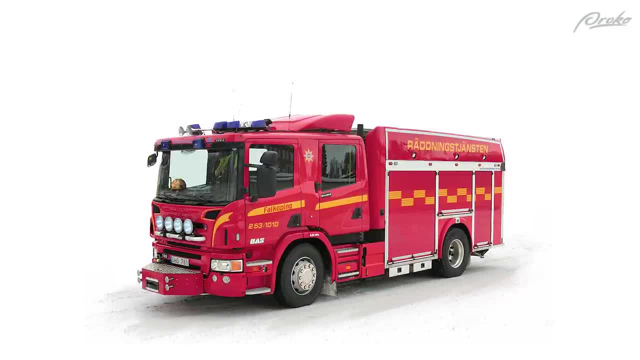 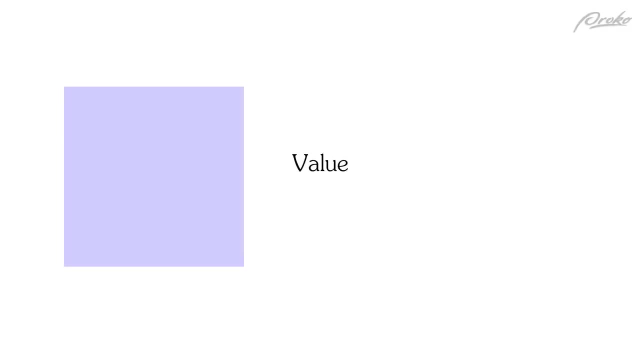 appears grayer. For an example, our fire truck features a more saturated red than a brick Which has a mid-chroma red. Now value- This is the one word that seems to trip everyone up. Value simply means how light or dark a color is. For an example, a light lemon yellow will have a 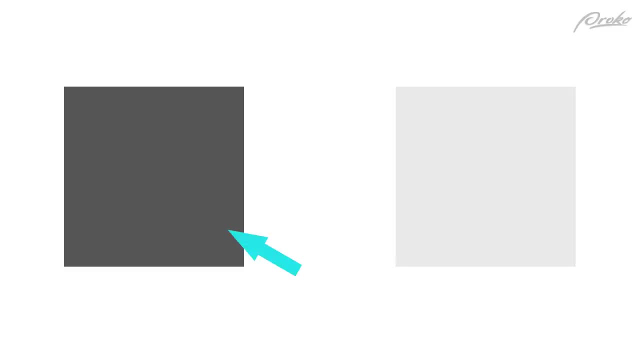 lighter value than a darker blue like ultramarine. Now, every color also has an inherent color temperature, meaning it leans closer towards the warmer side or the cooler side. We will get into that a bit later. This is the best way to define color, hue, saturation and value. It's the best way. 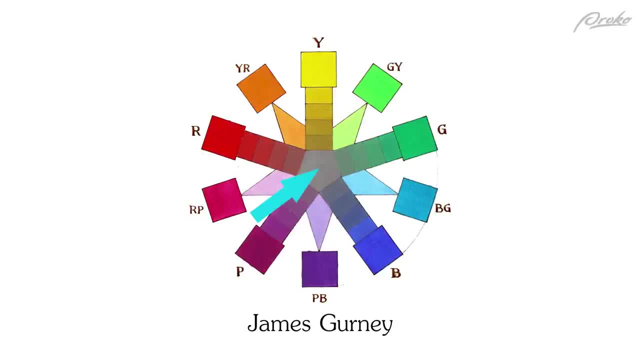 to define color, hue, saturation and value. It's the best way to define color, hue, saturation and value. This is the basic color wheel, which shows neutral gray in the middle and the highest saturation of the color at the rim of the wheel, which means there are a lot of neutral grays. 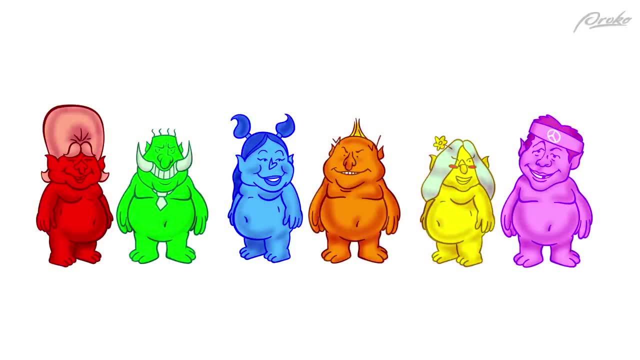 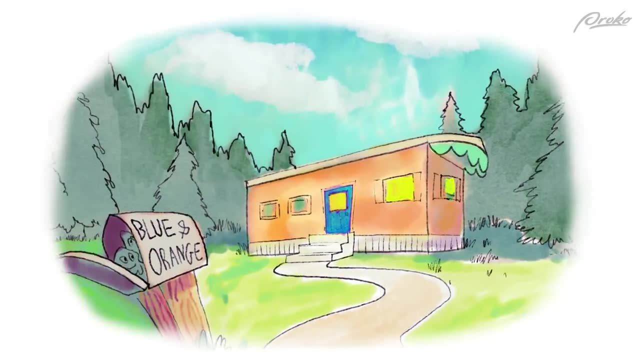 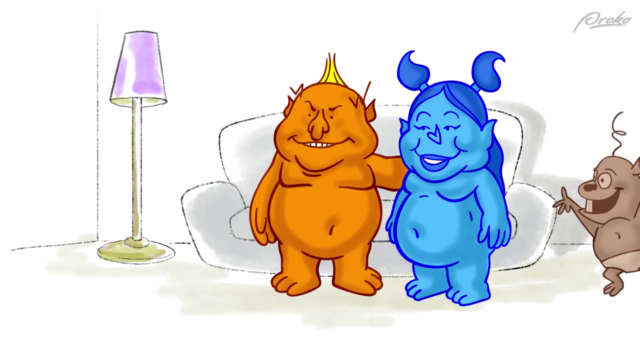 in between. I like to mix more desaturated colors from complements like red and green, blue and orange and yellow and violet. As you can see, you're basically mixing a primary color and a secondary color to get the best of both worlds and find all those beautiful. 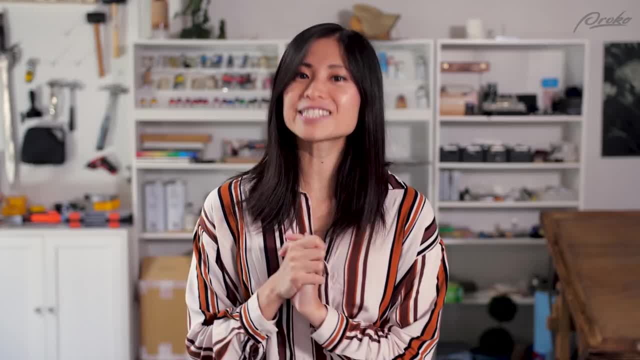 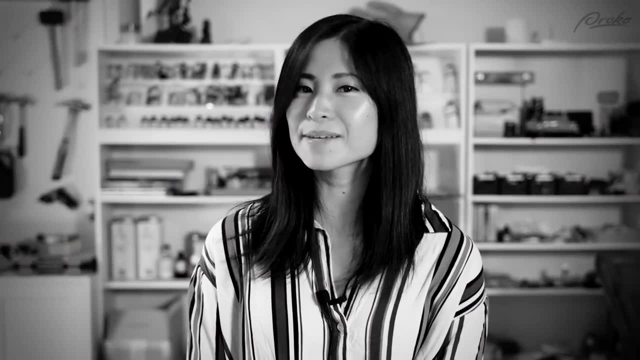 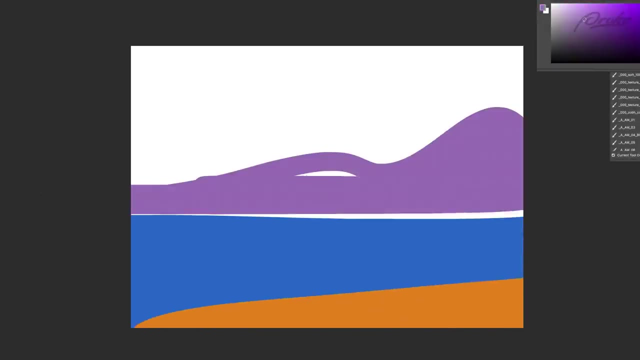 grays in between. I love injecting grays into a painting, but we'll get into that later on in the video. For now, let's put in our detective hats and go debunk some mysteries on color. shall we First debunk? If you think you have the wrong color, chances are you have the wrong value. Yes, you. 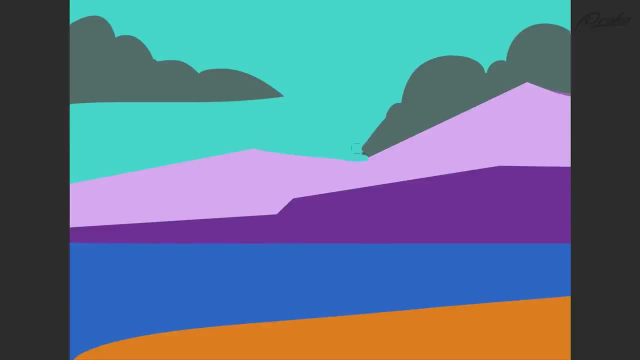 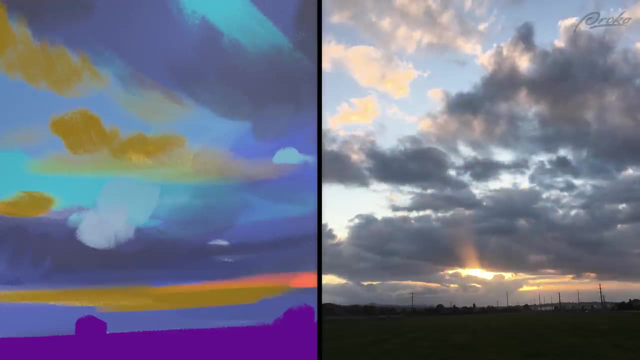 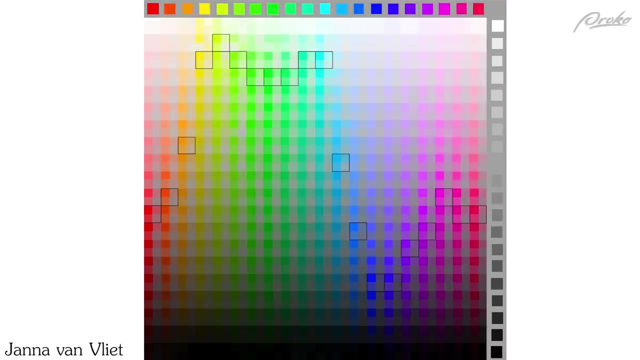 heard me right. 90% of the time, when a painting is not looking right and the mood just isn't pushing through, stop and act And ask yourself: wait, are my values working together the best that they can? Here's the thing. each color comes with an inherent value, which means that each color 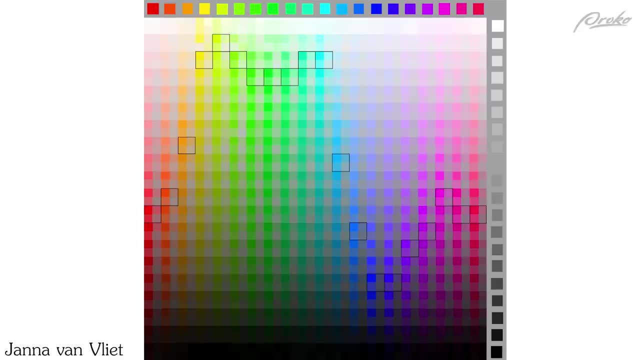 has a certain lightness or darkness. Here's a chart that one of my students made on her own to explore the different inherent qualities of 20 colors or hues. As you can see, yellow and green reach its highest saturation or chroma at a relatively high or light value. 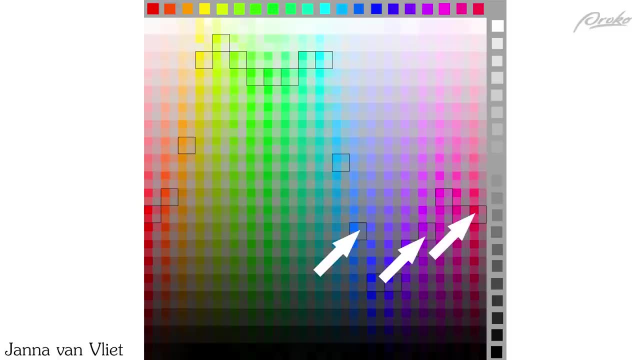 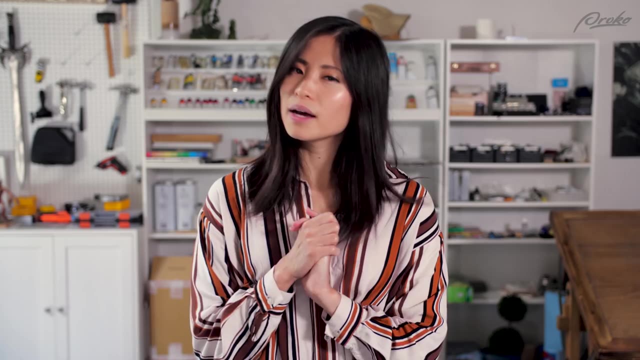 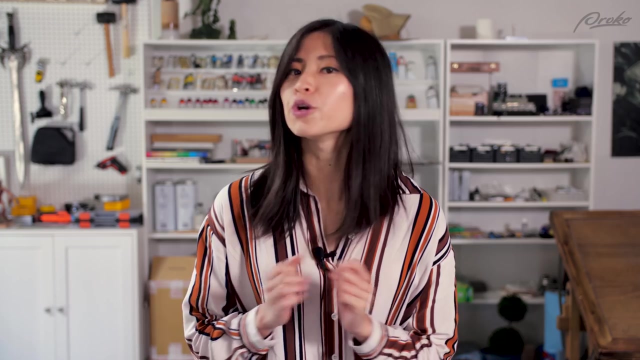 while red and blue reach their highest intensity at a lower value, Every color is completely unique. Now, since there are so many colors out there, it's important to train your eye to see if the values of the colors you're putting down are working with each other in a painting. 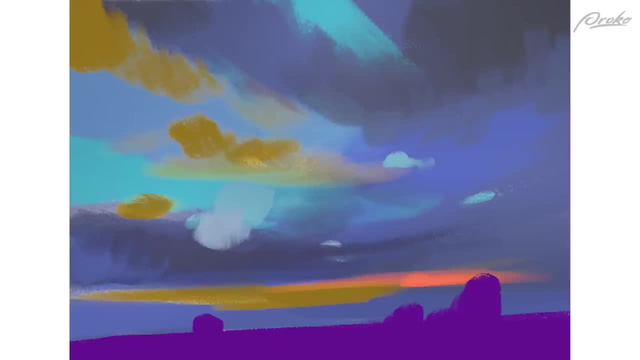 What can happen is that your painting can look really pretty on the outside with all those happy, more saturated colors, but when you turn it black and white it falls apart and just doesn't read well. Kind of like a dry, crumbly cake, only held together with. 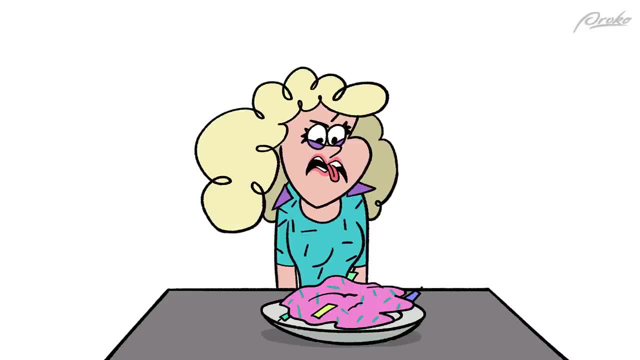 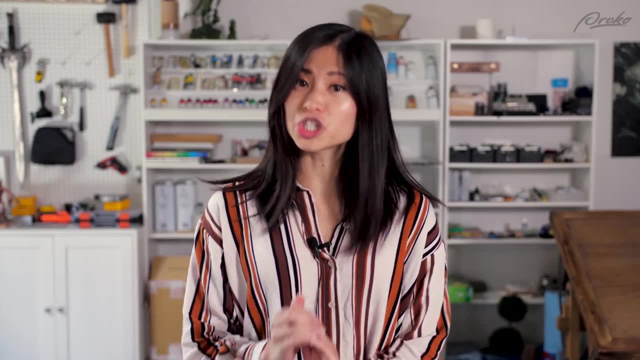 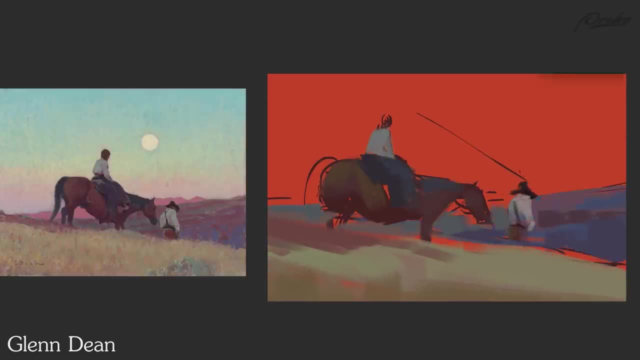 extra sugary frosting. Now, who wants that Second debunk? There's no such thing as a muddy color. They're only muddy relationships of color. Don't like gray, Don't like brown. Well, there are so many kinds of grays, browns and earth colors. Using those colors can sometimes be the best way. 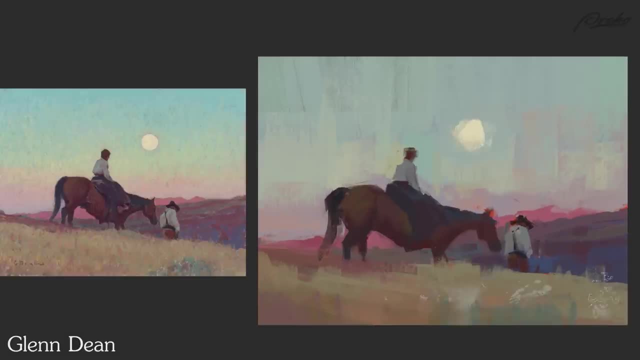 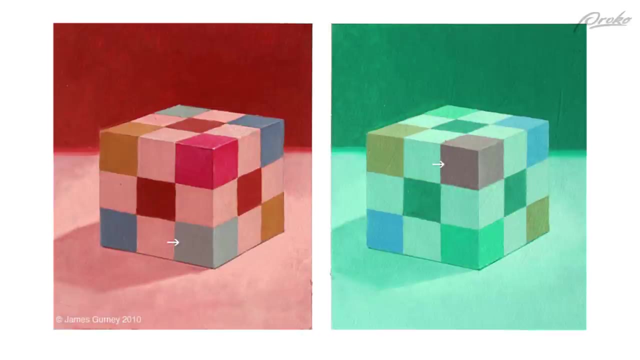 to accentuate your pops of color. You can also use them to color up your painting when you use those colors right along your more saturated colors, because they act as supporting actors to accentuate your pops of color. Colors are relative and exist in relationships, so something. 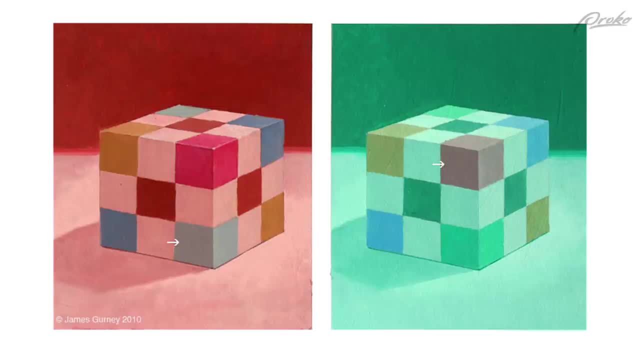 that might seem like a boring gray on your palette can look completely different when you add it into your painting, because the surrounding colors influence how that color looks, proves just that. Can you tell me what those colors that the arrows are pointing to are, Those two squares of both images? 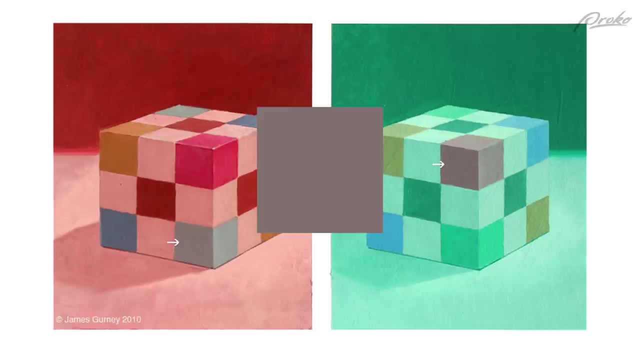 are in fact the same color. If you don't believe me, let's just take this gray square and place it in the exact same spot on both cubes. Now you can see in real time how your eye is playing tricks on you. The 50% gray on the left: 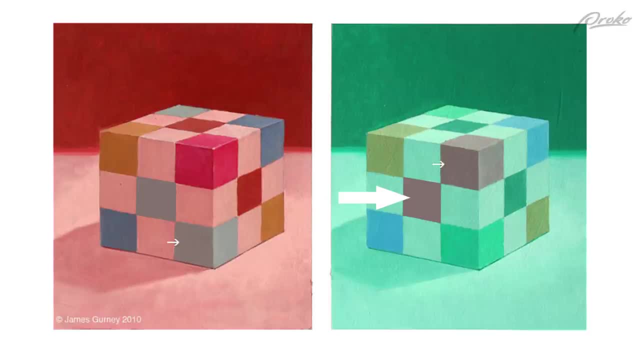 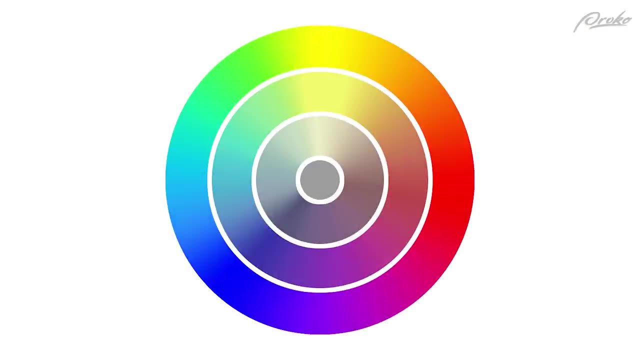 starts to look like a greenish gray, and the same gray on the right starts to take on a reddish tone. But there's more. Remember when I said there is not one kind of gray. There's a whole world of grays waiting to be explored. 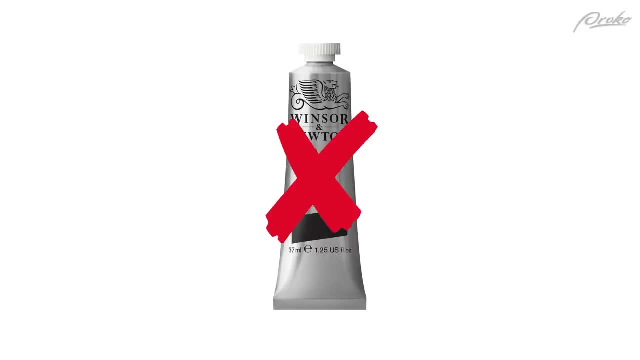 So let's dig right in. I personally never use black when I'm trying to darken and desaturate a color, But that doesn't mean that you can't use black. Sometimes using black is in fact necessary to get those nice, dark, rich tones. 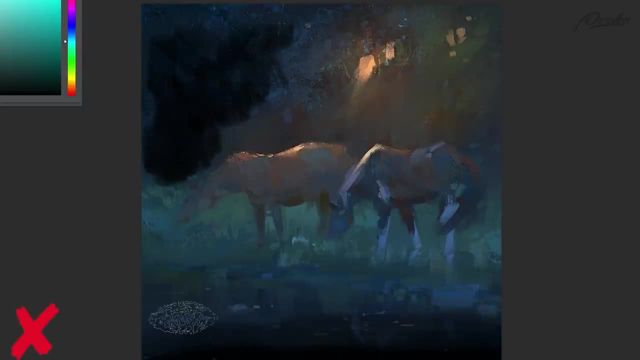 If you do use black, the tip is to never just put straight black or white in your painting unless there's absolutely no other way. In my experience, those colors just don't vibrate with other colors as much and oftentimes will flatten out your painting. 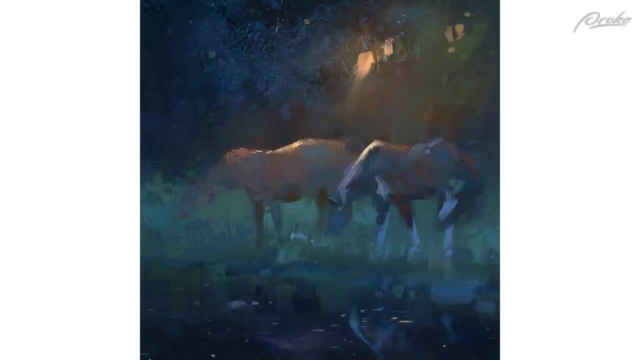 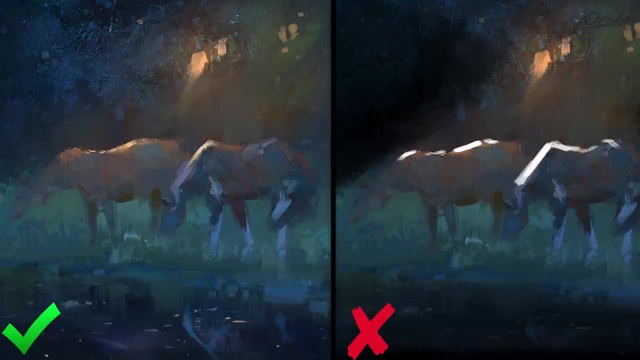 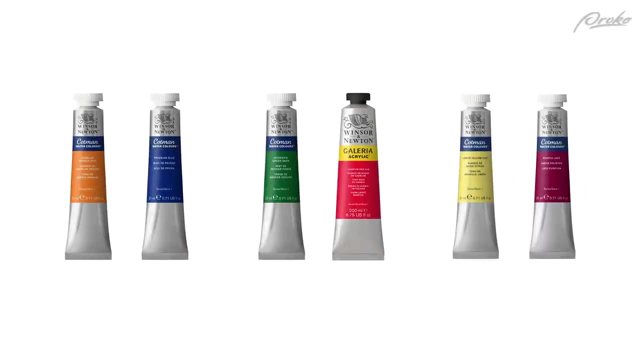 Mixing black with another color, such as red or blue, will assign it a color temperature, thereby shifting your darkest values just slightly warmer or cooler, and add a subtle richness to your painting. I personally like to use complementary colors to mix my grays and darken my colors. 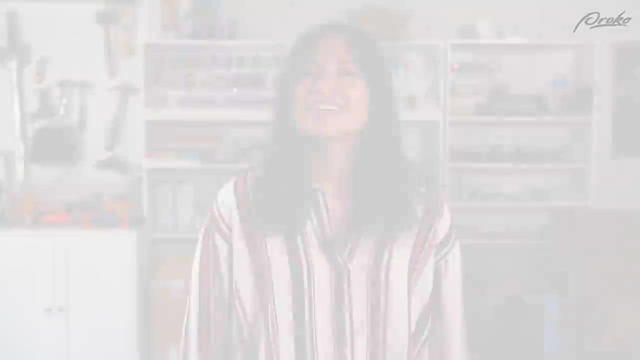 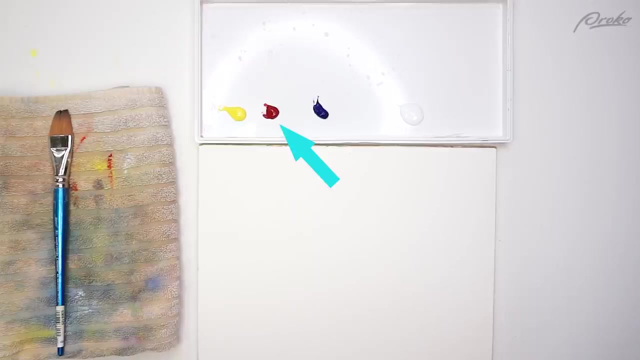 but still get a full range of color within my painting. So if you're scratching your head, I'll show you what I mean. On my palette here I have the primaries: alizarin, crimson, ultramarine, lemon, yellow and white. 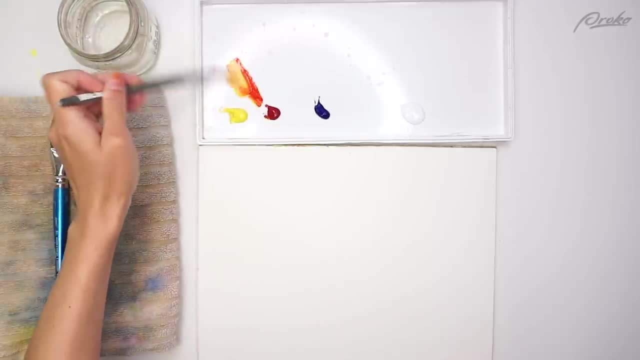 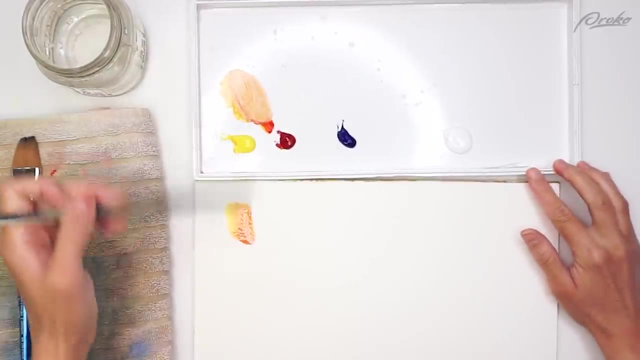 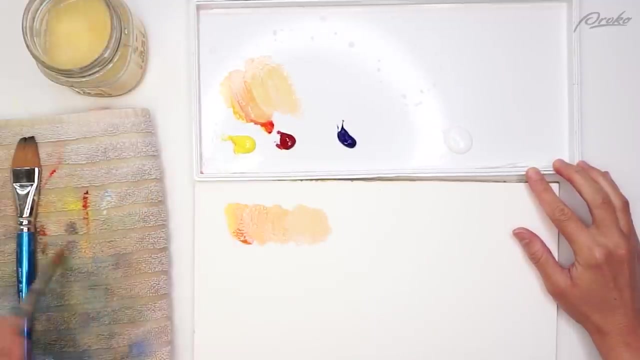 Let's see how we can mix the secondary colors, first from these primaries. To get orange, I'm mixing alizarin crimson with lemon yellow. As you can see, mixing in white gradually lightens but also cools down the color. It is important to remember that white desaturates. 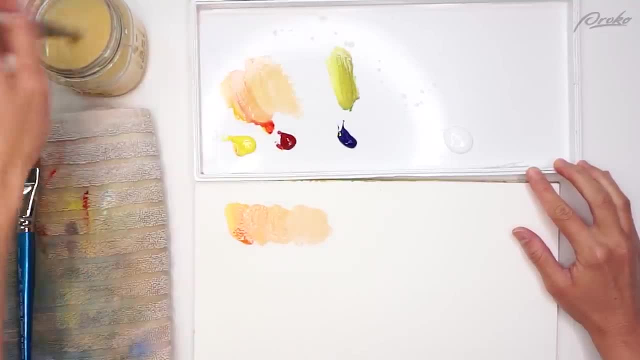 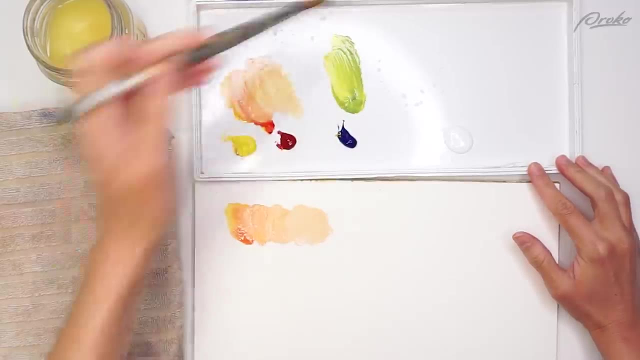 which means that you're stripping down the chroma or intensity of a color. the more white you mix into it. Now, to get green, I'm mixing ultramarine with lemon yellow. The more yellow I mix in compared to blue, the warmer and lighter the green will get. 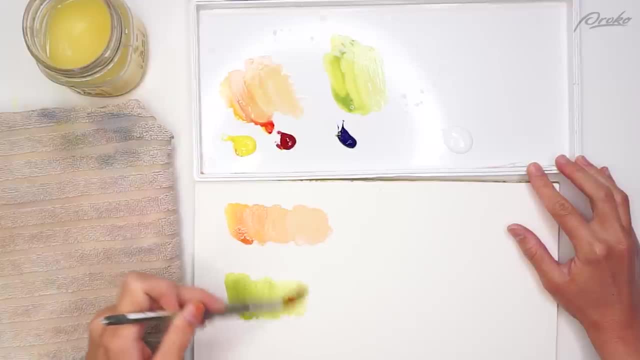 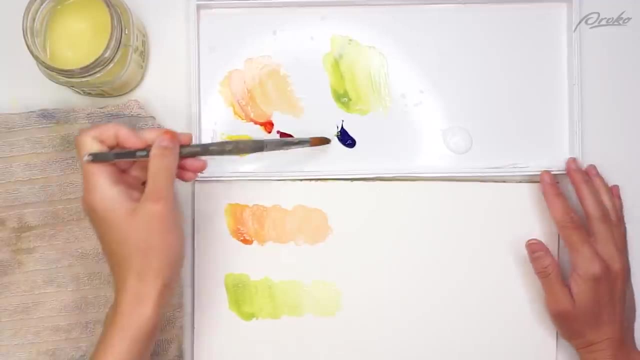 because yellow is a warmer and lighter color. If I mix white into that green, I'm also lightening and cooling down that green. Now, as you can start to see, the more blue I mix in compared to yellow, the cooler and darker the green will get. 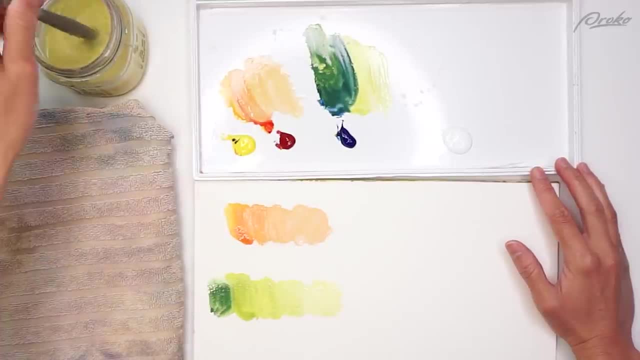 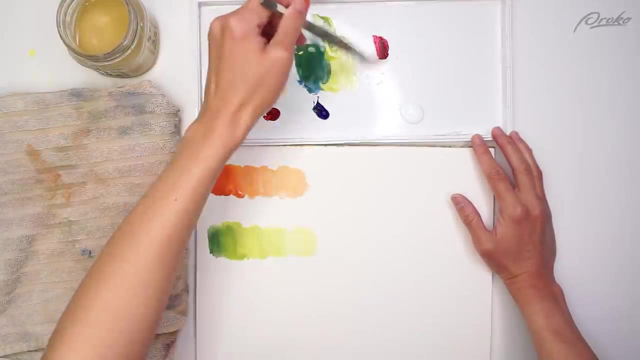 because blue is cooler and darker than yellow. Do you start to see how many greens of varying color, temperatures and values you can get with just two colors? Lastly, let's mix the violet. I'm mixing one with more red and one with more blue. 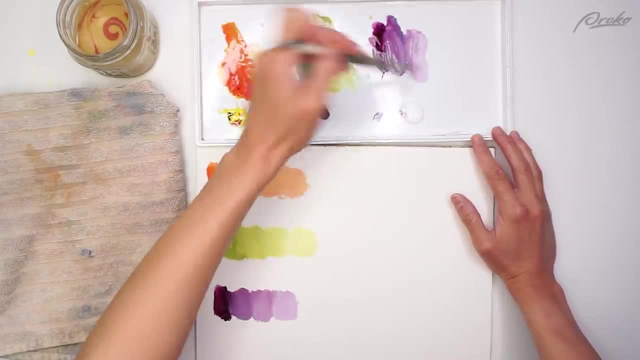 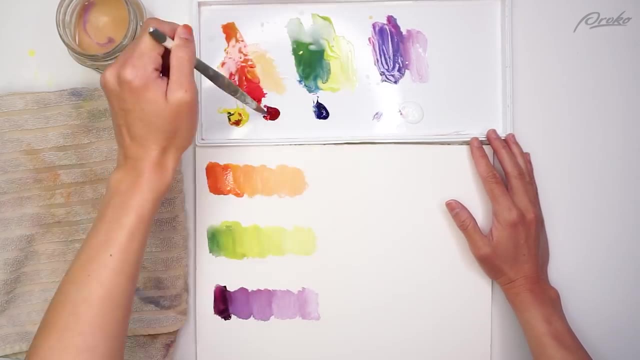 Let's see how we start getting warmer and cooler versions of the same hue family. As usual, mixing white lightens and desaturates. Now that we have our secondaries, we can mix the primaries and the secondary colors together to get our neutral grays. 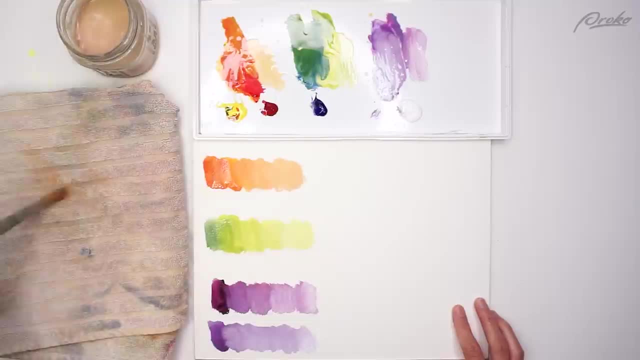 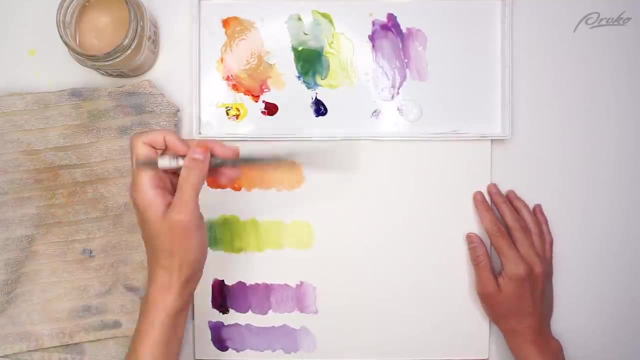 Watch what happens when I start mixing a bit of blue into the orange at the top. Just by incrementally adding a bit more blue and white each time, I'm desaturating the orange and lightening it up at the same time. With practice I can get a beautiful spectrum. 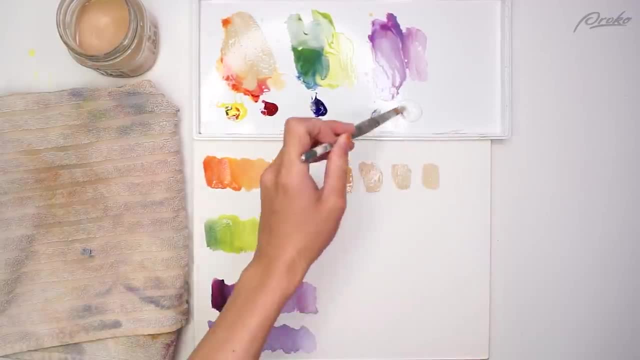 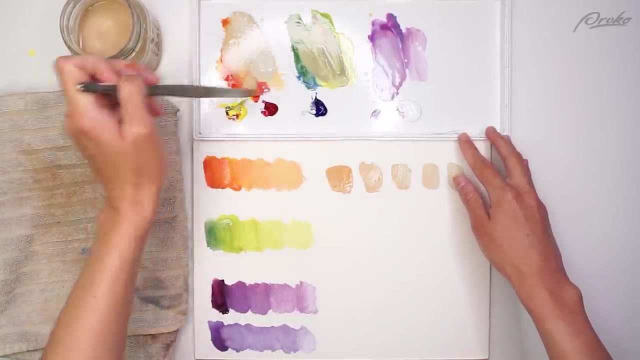 of bluish grays or warmer grays that carry a tinge of orange. The same happens when I start to mix a bit of red into the green, Depending on how much red or how much green I mix in along with white to lighten if needed. 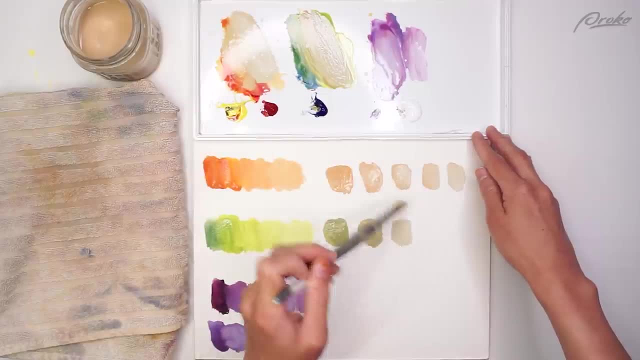 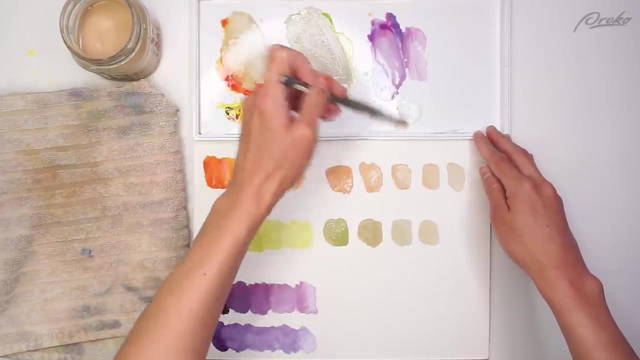 I start getting warmer reddish grays or cooler greenish gray. If I start to add white, I'm cooling down these grays even more, while lightening at the same time, thereby giving it a little higher or lighter value. Lastly, let's do the same with violet and lemon yellow. 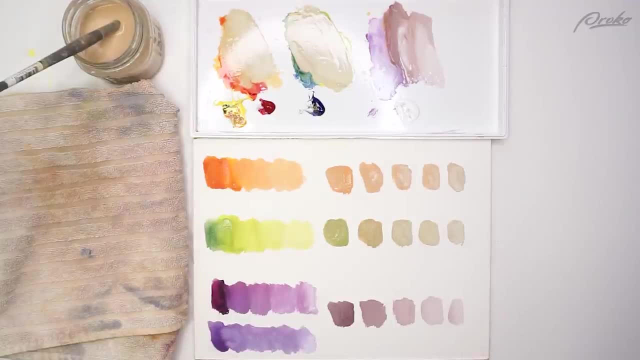 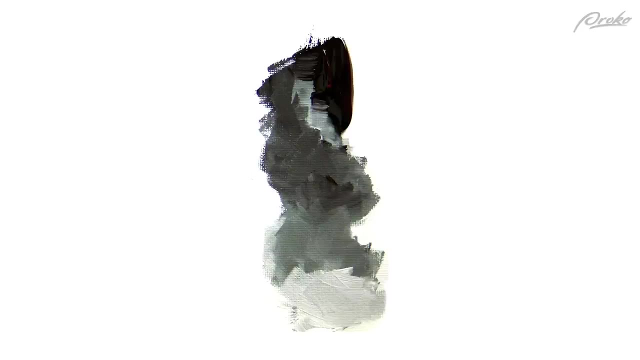 Can you see how we start getting a beautiful picture just with these grays, Now that we've established that there's a whole world of neutral grays to be explored? it is safe to say that there is not one kind of gray, simply mixed from black and white. 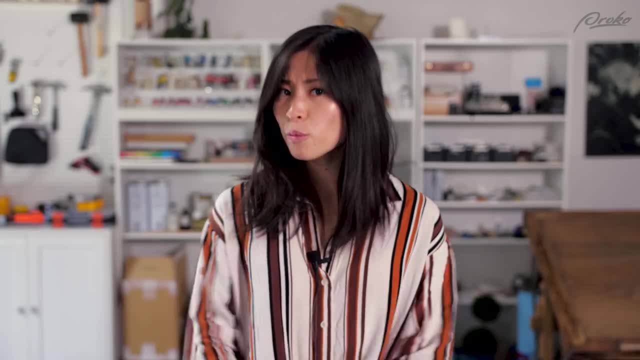 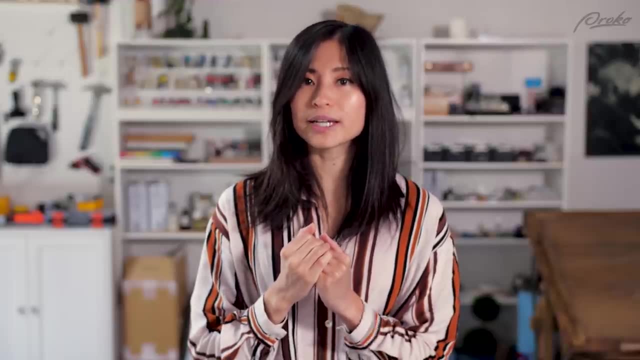 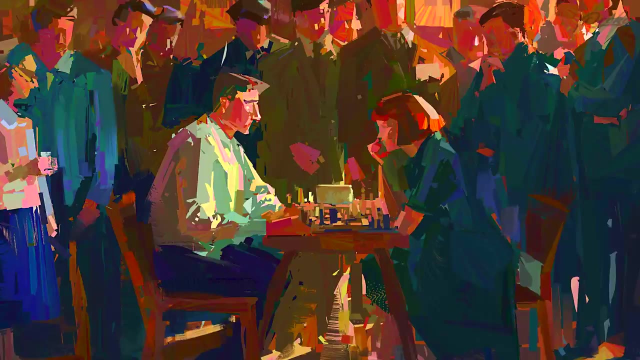 Now you're probably wondering why are neutral grays so important to put into a painting? I like to think of them as a supporting actor that are necessary to accentuate and support your bolder, more saturated colors in your painting. If your painting only had saturated colors everywhere. 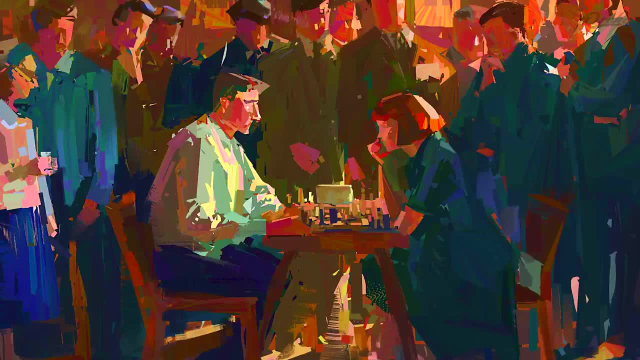 they would be competing with each other like 10 babies crying and nagging in a room. Grays in a painting help bring balance and harmony, and that's why they are so essential. I love what Charles Hawthorne has to say about grays. 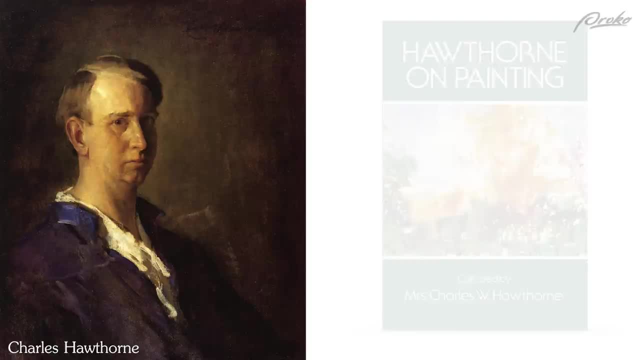 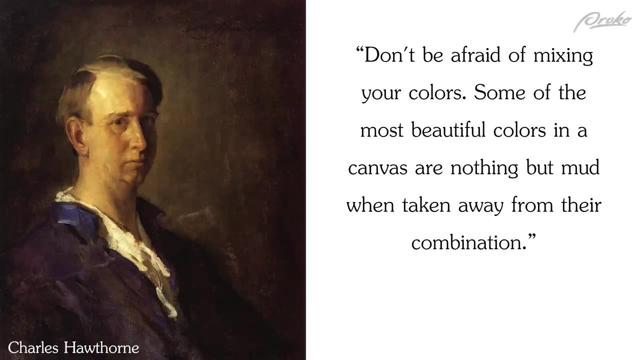 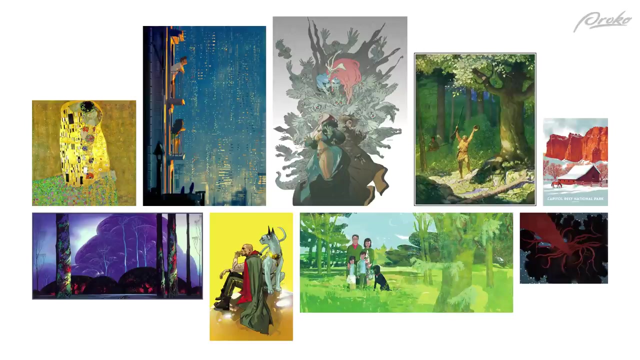 in his book On Painting, in which he explains that the mud he mixes from this palette can completely transform when you put that mud into your painting. Remember colors exist in relationships and colors that are mixed on a palette will take on a whole new identity. 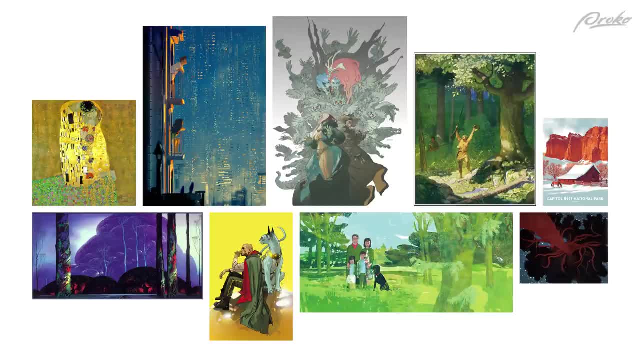 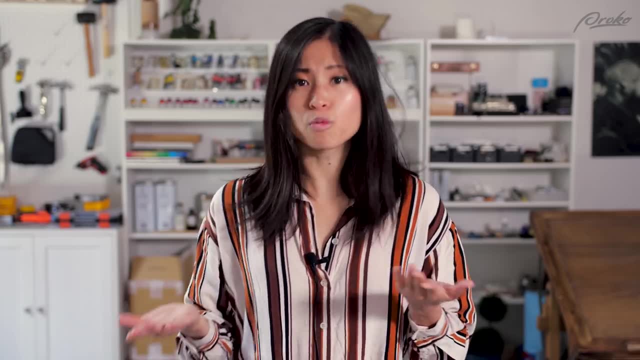 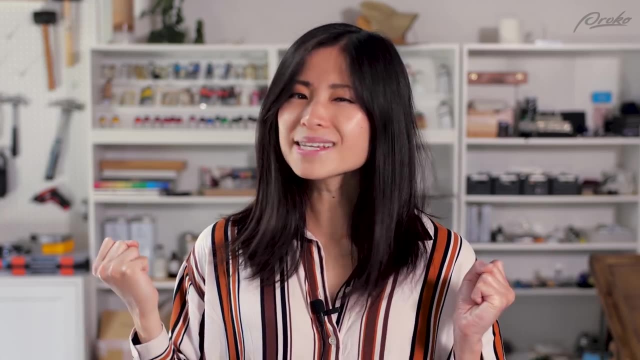 when you put them on the canvas alongside other colors. Third debunk- So you've probably heard it many times- Red and yellow are warm colors and blue, purple and green are cooler colors. So this is true to an extent, but why such definite labels? 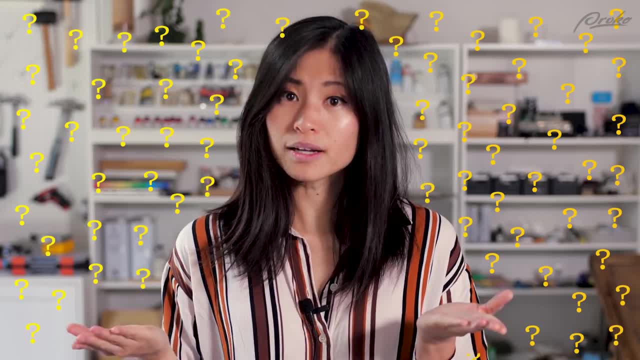 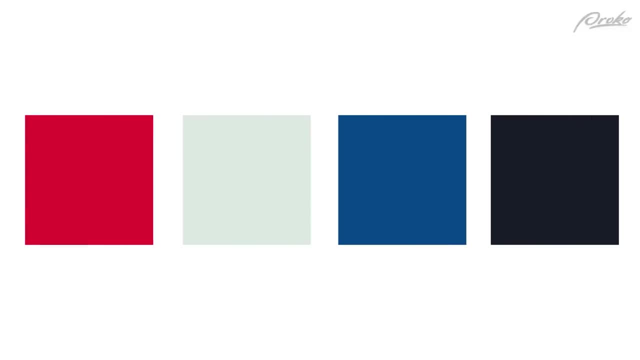 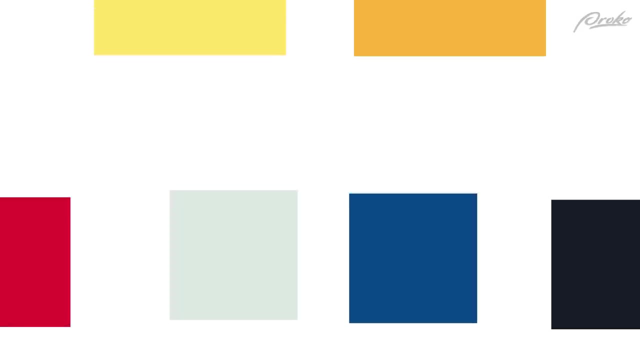 Maybe you're wondering: can yellow be warmer and cooler? And the answer is yes. I dislike blanket statements like this because to me, it limits your imagination. It's easy to say: oh yes, red is clearly warmer than blue, which is correct, but what if I put two yellows side by side? 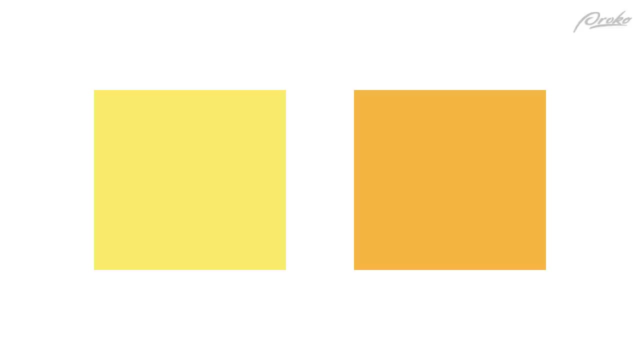 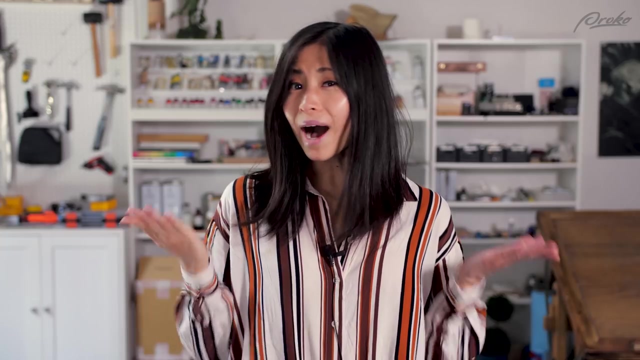 Now, can you tell me which one is warmer? Did you figure it out? The answer is the right one: Permanent yellow, deep is in fact a little warmer. Why? Let's go back to the mixing board to find out. Now, here I have lemon yellow squeezed out. 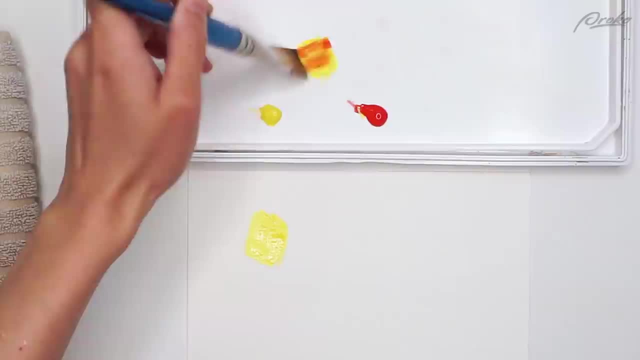 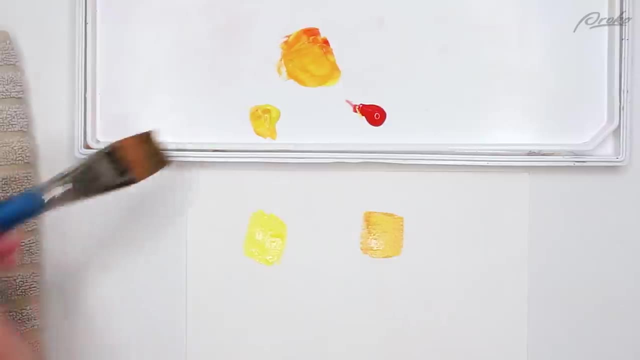 To make it warmer I would need to mix a teeny amount of alizarin crimson to warm up the yellow to make it closer to the yellow I had earlier- permanent yellow deep. By mixing in a bit of red I'm making the color even warmer and slightly darker. 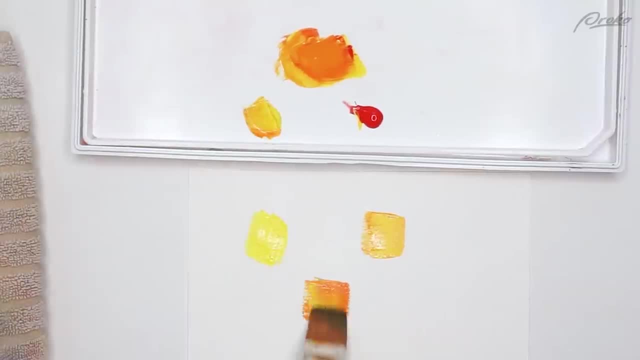 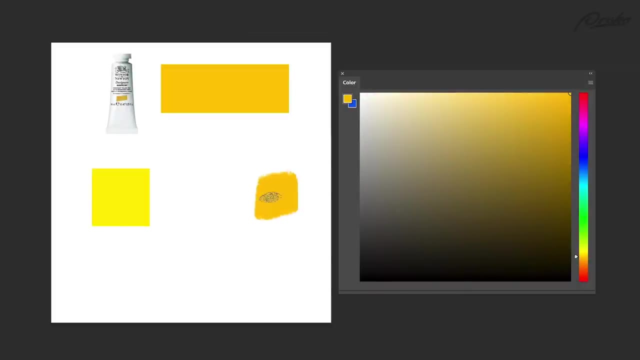 than it was before, because red is a warmer color, while lemon yellow has a bit of green mixed in. If we shift over to the digital hue box, you can see this as well. If I'm trying to match a permanent yellow deep from a lemon yellow. 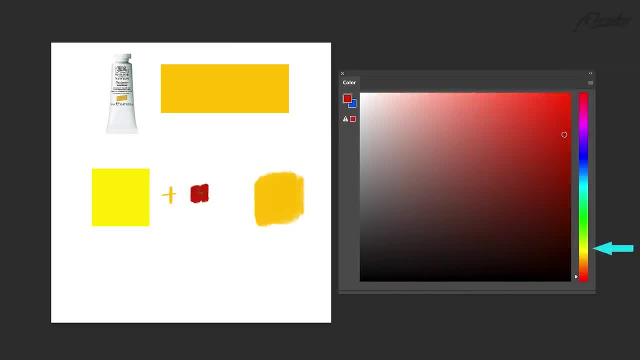 which is a cooler yellow than its former, I have to move the slider down towards the reds to get a warmer yellow. Similarly, if I want to warm up a cooler cobalt blue and make it more ultramarine, which is a warmer blue, 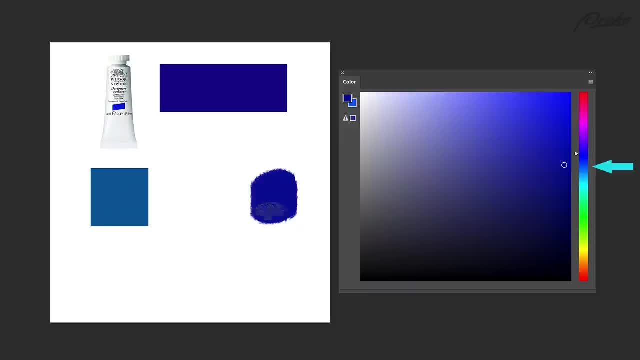 because it has a bit more red mixed in. I'm now moving the slider up towards the magentas and therefore adding a bit of warmer red into the mixture. Traditionally, I would be mixing alizarin crimson as well to warm up the cobalt blue. 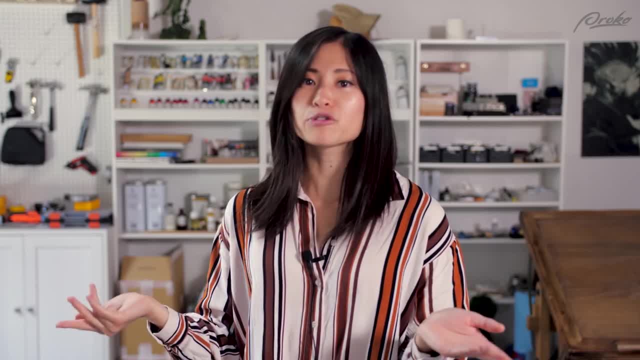 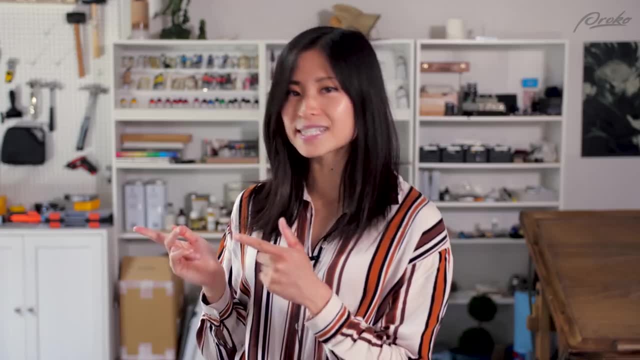 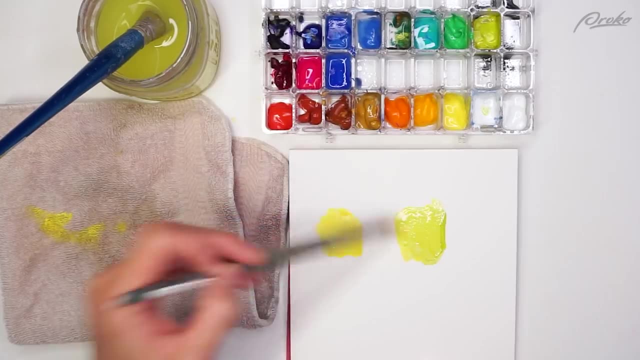 Fourth debunk: Happier, warmer colors are always lighter than cooler colors, but is that always the case? Let's head over to the mixing station to find out. I'm going to take a warmer color, like permanent yellow deep, and compare it to a cooler color like linden green. 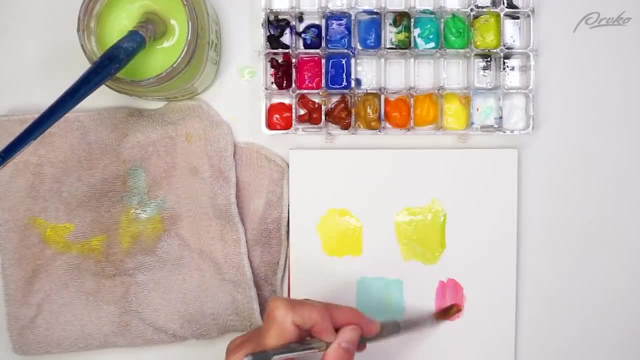 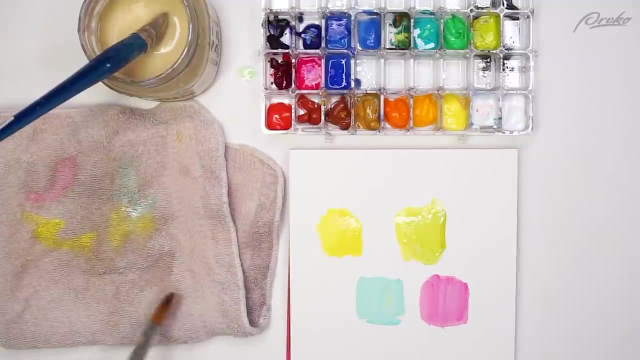 Let's do something actually a bit more obviously opposite, like turquoise and magenta. The goal here, however, is to get these two colors to be the same value. Now let's turn this black and white. Do you see how the value difference? 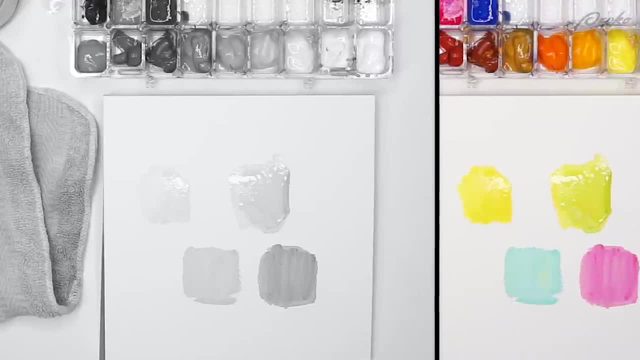 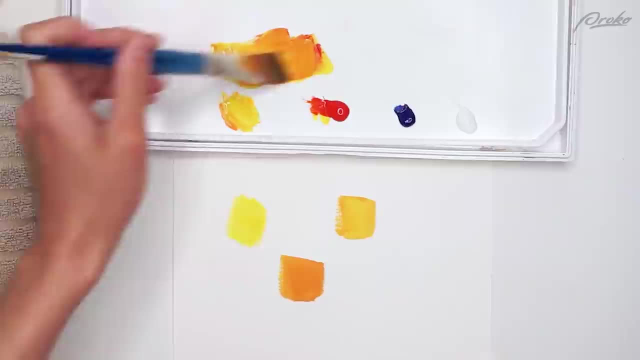 is actually not that big between the colors, even though one color is clearly warmer and the other color is clearly cooler. Let's see. Now let's do one more example. I'm going to mix a darker, warmer color- alizarin crimson- with the yellow. 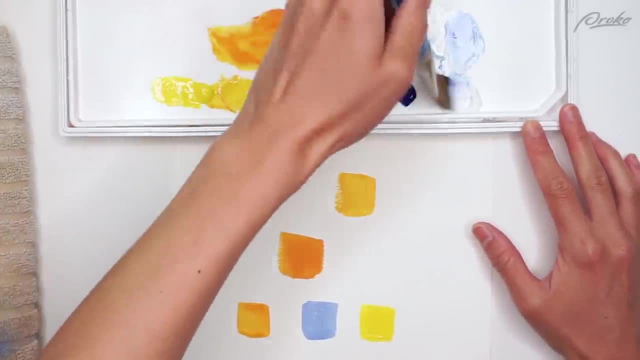 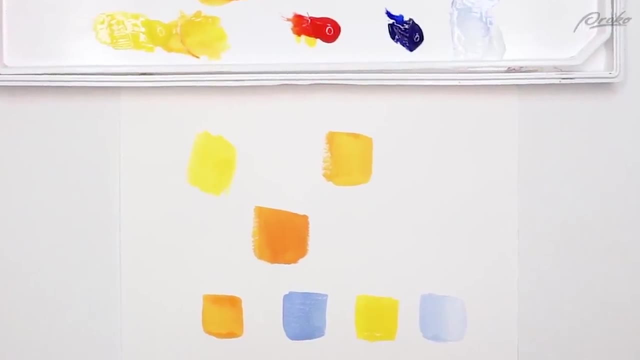 to darken that yellow a bit more and warm it up. Now let's mix a bit of white into the cobalt blue just to lighten it up. Both colors are still maintaining their relative color temperature- warmer and cooler. but when we turn it black and white, 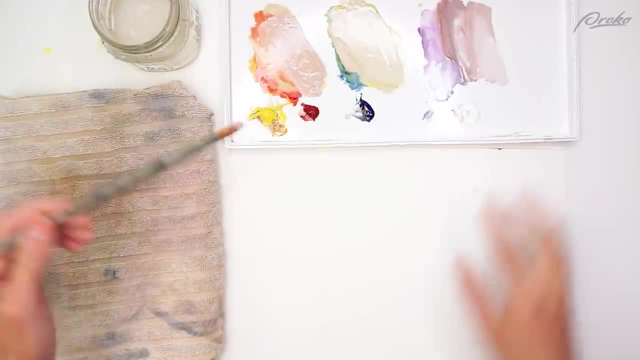 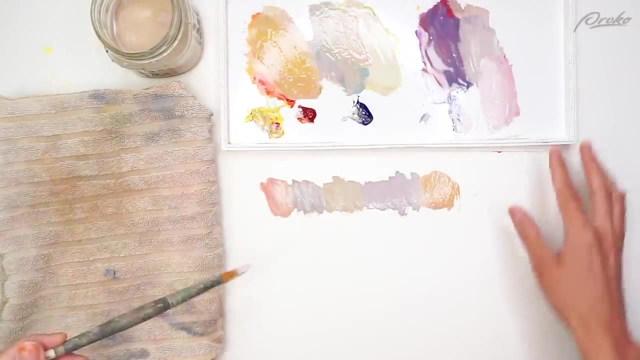 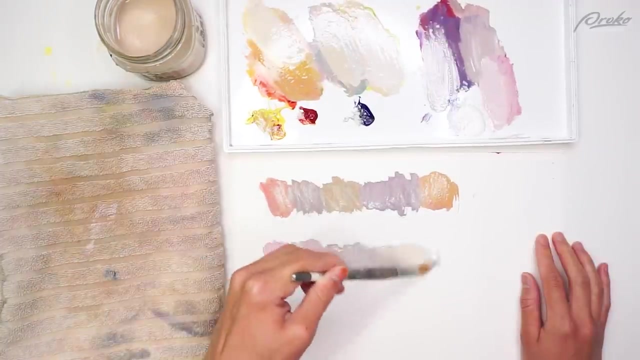 they're almost the same value. Now, taking that concept, you can indeed combine colors of varying color temperatures and saturation while maintaining the same value, which I believe is key to creating variety in your painting. The goal here is to practice, training your eye. 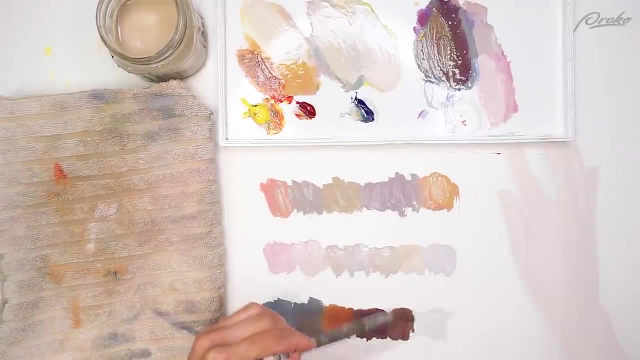 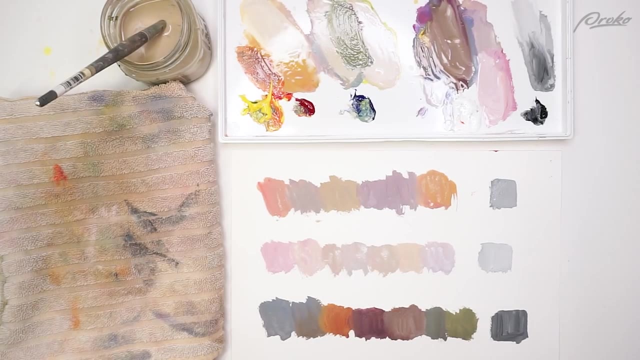 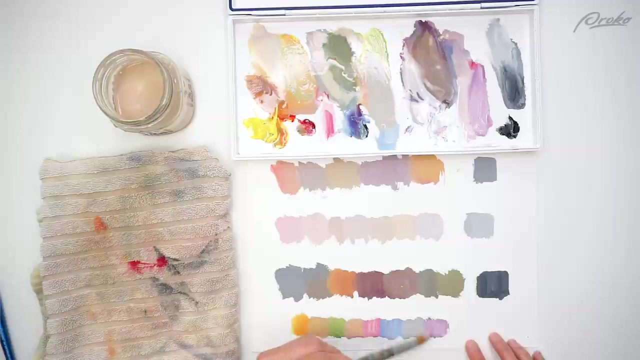 to mix colors of the same value so that you can get variety and contrast in your painting, not through value but through subtle color temperature shifts. Now, with a bit of experimenting, you've gotten a lively combination of colorful grays with more relatively vibrant colors. 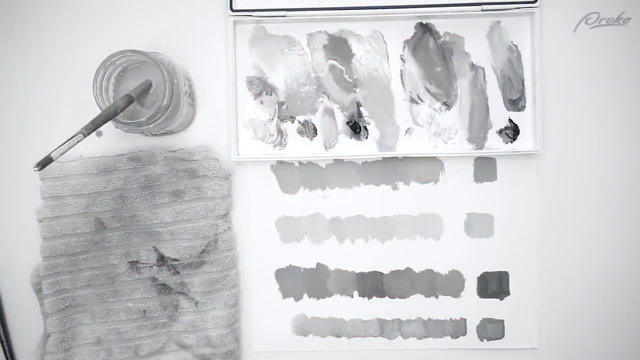 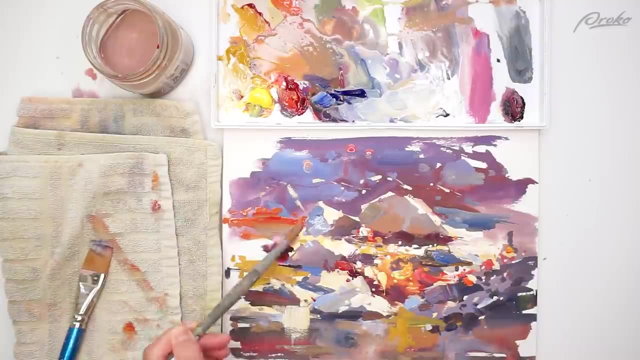 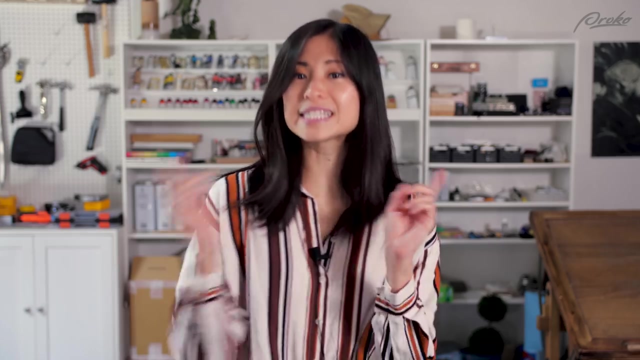 that all have similar value. And why is this so valuable, you ask? Because this is how you get beautiful color shifts within the shadow and light shapes of your painting, while maintaining a readable and strong value structure as your foundation. Now let's head over to the digital hue box. 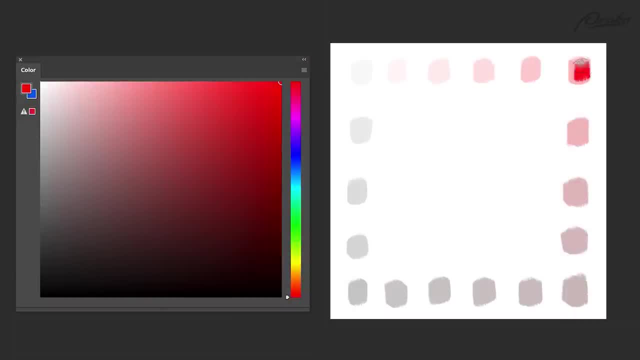 to understand this more. In this hue box in Photoshop, the top right corner is where the color is at its highest saturation, or chroma. As you drag your color picker down, you are decreasing in value, In other words, you are darkening the color. 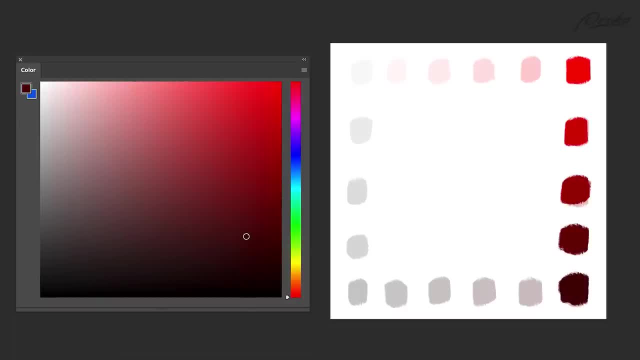 and thereby making darker shades of that color. As you start moving your color picker over to the left, you're entering into the realm of grays. On the very left side of the square is grayscale As you start moving your cursor away from the very left edge. 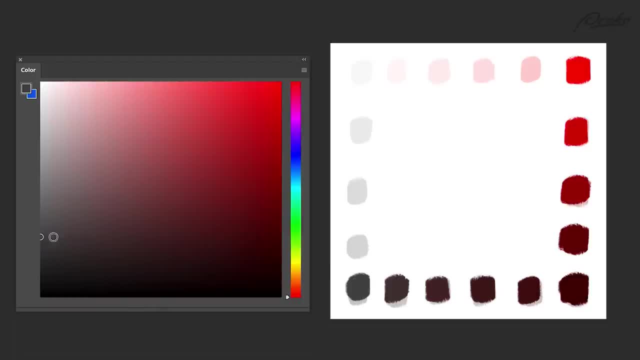 you start getting all kinds of beautiful, warmer and cooler grays. If you move your cursor up, you're essentially mixing white in and lightening and desaturating, as white always lightens and cools the color. Then, as you make a full circle, or square in this case, 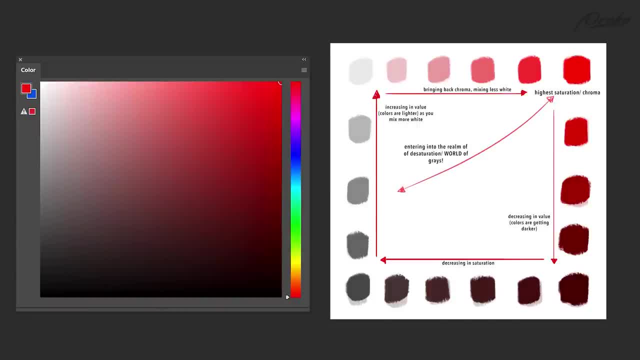 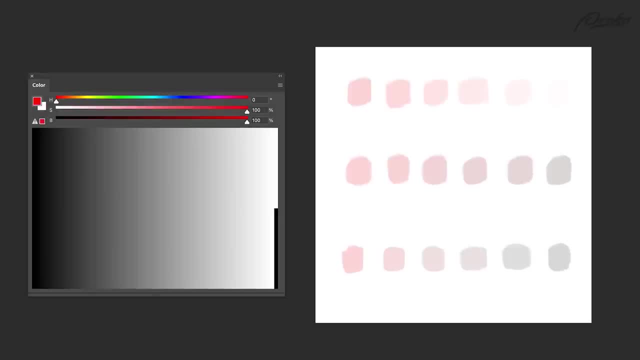 and drag it along the top edge of the box, you're slowly bringing back the saturation, with more pigment and less white. Now let's shift over and explore another way to look at this. Let's look at HSV or HSB sliders, which stands for hue, saturation and value or brightness. 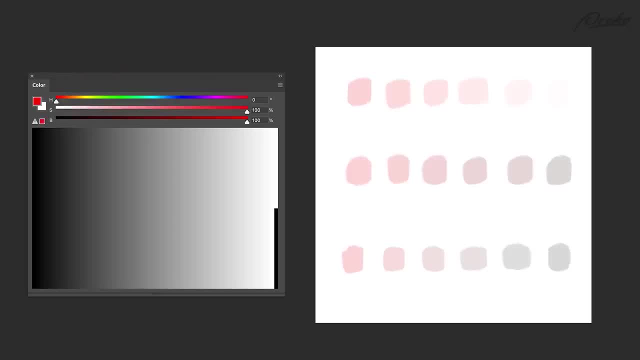 On the top slider we are choosing the hue that we want. The highest saturation or chroma will be when the saturation slider and brightness slider are both nestled on the very right. Let's play with keeping the brightness or value in the same location at the very right. 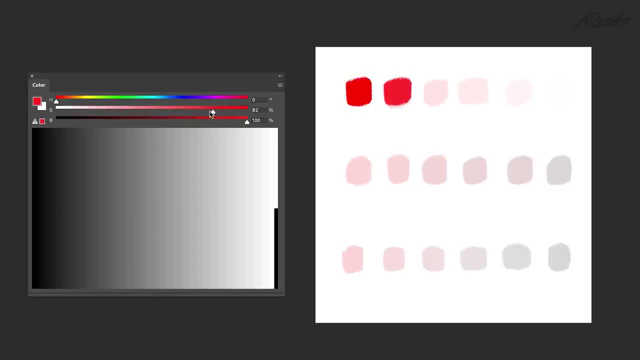 but play with moving the saturation slider. By moving the saturation slider incrementally to the left, we are essentially mixing more and more white to desaturate the red Because, remember, white always desaturates, lightens and cools, Since the brightness is being kept at the highest level. 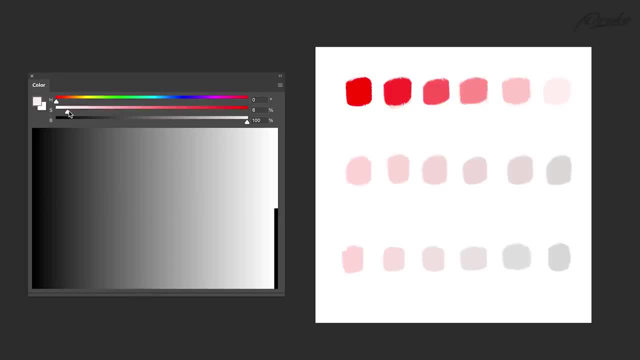 the color gets lighter while the saturation decreases. Now let's reverse that and keep the saturation slider at the very right, but move the brightness slider incrementally to the left. You can see now that we are darkening the value while maintaining relative saturation. 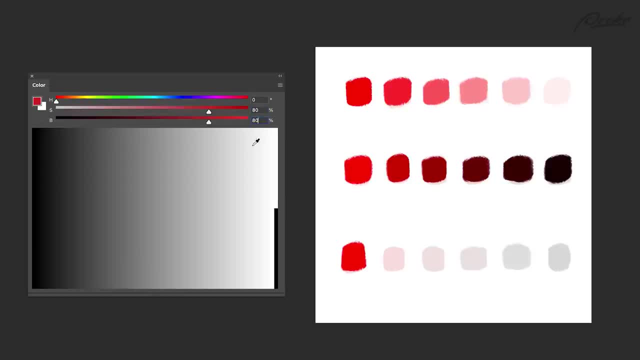 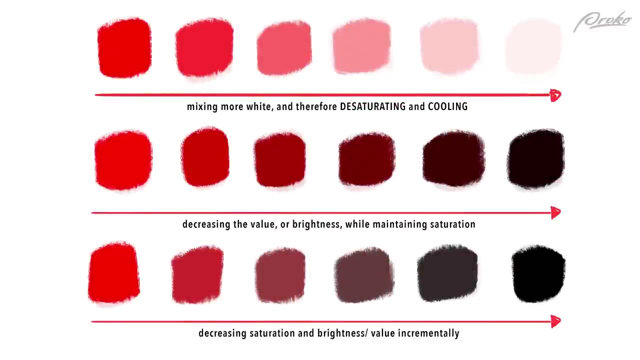 Now, if we start to move both sliders to the left incrementally, we are decreasing the color's chroma and value, thereby getting more grays with darker and darker values. Adjusting the sliders might seem tedious at first, but it really helps you deconstruct and understand colors. 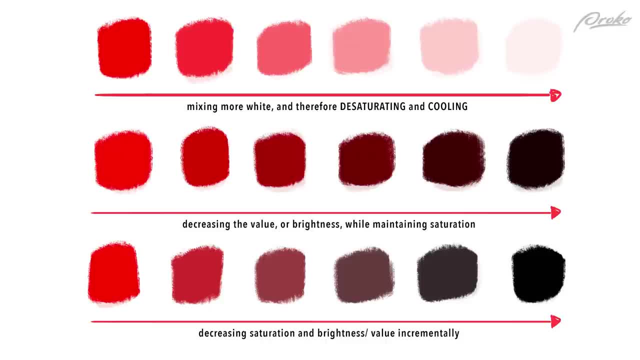 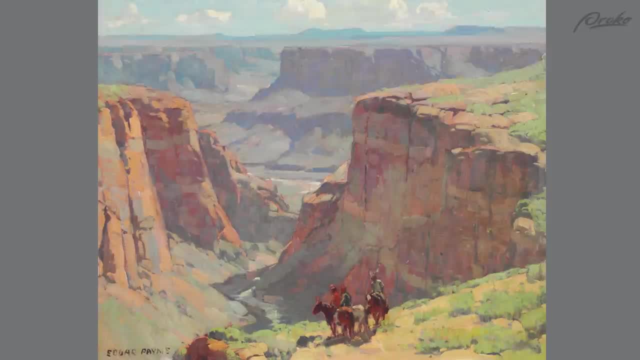 in a more mindful way than just simply color picking from a photo? Do you start to see the myriad of combinations you can have when you incrementally break colors down this way? Let's apply everything we've learned in this case study of this beautiful painting by Edgar Payne. 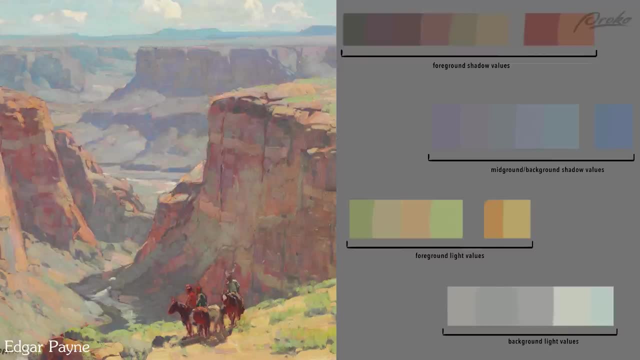 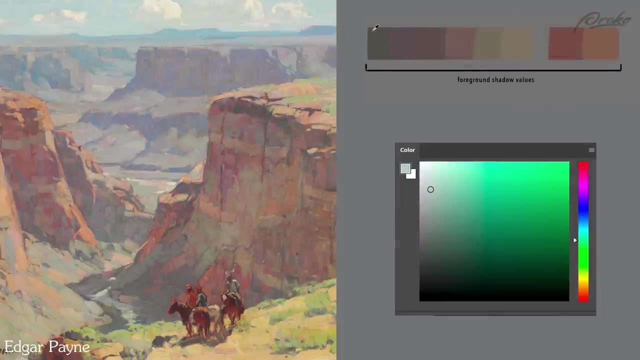 called Writer's Overlooking Canyon. The value structure of this painting showcases a darker foreground graduating into a lighter background. I've broken down the shadow family colors and the light family colors against a 50% gray background on the right. On analyzing the color relationships, 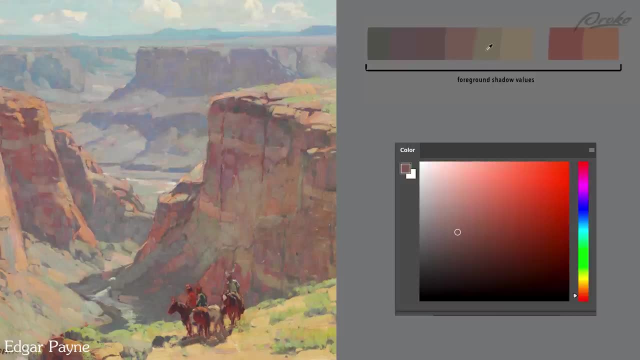 you can see that the shadow and light family. you can see that the cliff shadows exhibit a myriad of warmer tones in the red and yellow hue family. But within those colors, Payne is playing with different levels of saturation in reds and yellows, while maintaining similar value. 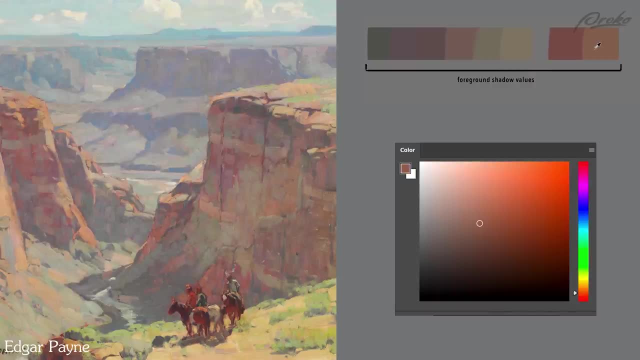 In other words, he's playing with different levels of more saturated reds and more grayed reds and yellows to get a beautiful combination of color just within the shadow area in the background of the cliffs. Now in the shadow shapes of the background cliffs. 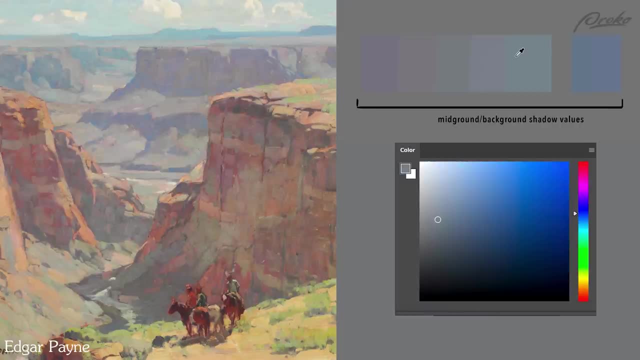 you can see that the values have gotten lighter, cooler, because there are more blues, and more desaturated overall, with warmer and cooler blues sitting beautifully together. This is essential for creating that depth and atmosphere in the painting Now in the foreground, where the cliffs are being lit. 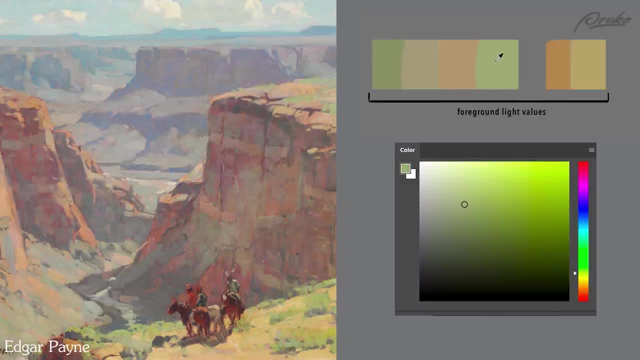 Payne is actually playing with some lighter and cooler colors compared to the shadow side. he is using some greens, yellows and oranges, but all are pretty desaturated in chroma. We know that because they're sitting closer to the left side of the hue box. 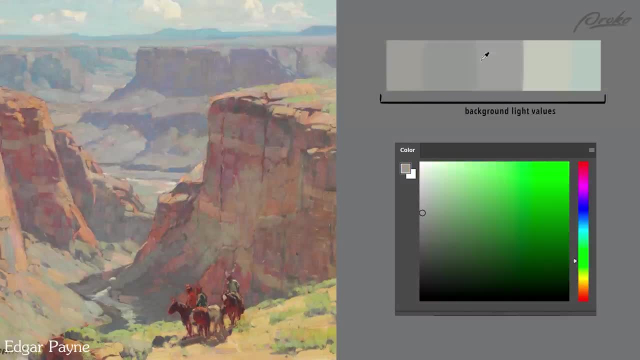 Lastly, for the lit areas of the cliffs in the distance, you can see that the colors, although they appear quite lively within the actual painting, are no more than fairly light grays hugging the very left edge of the hue box. However, within those colors, 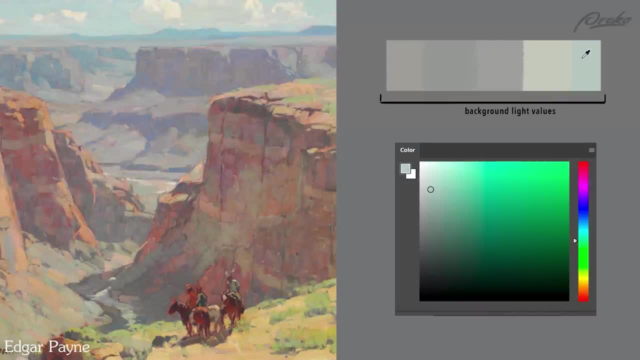 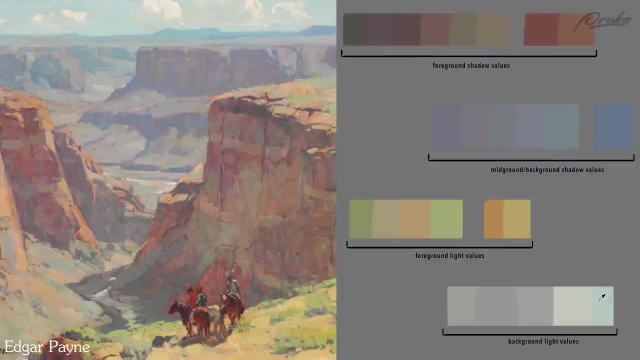 However, within those colors, you can see that we are still shifting ever so slightly in color temperature, with slightly warmer grays and slightly cooler grays. When we turn everything black and white, you can see how the value structure of the painting holds beautifully. 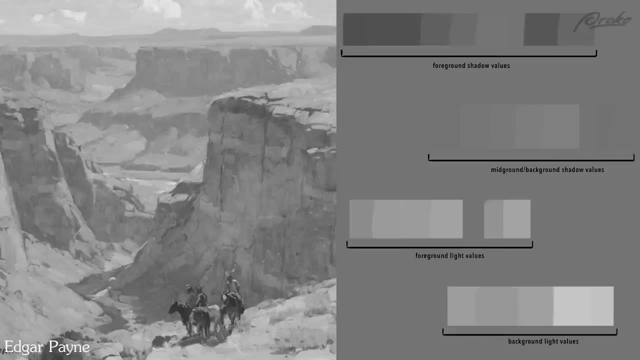 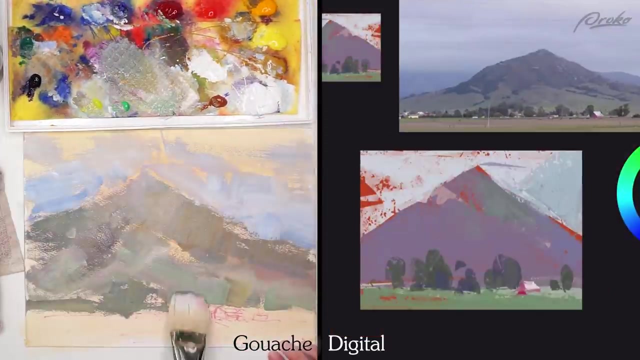 You can also see how the color swatches on the right in each group all have similar values, while shifting in slight hue and color temperature to get that beautiful variety. Now it's important to note that when you mix colors on a digital canvas like how you would traditionally, 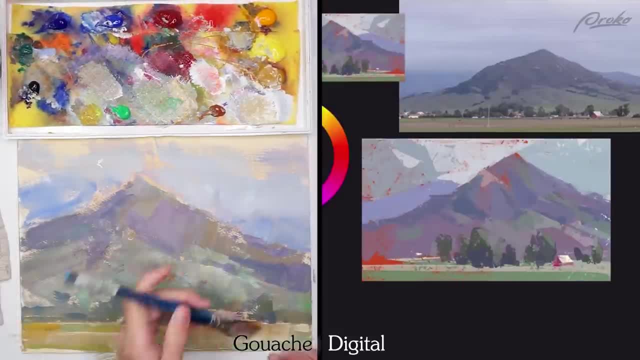 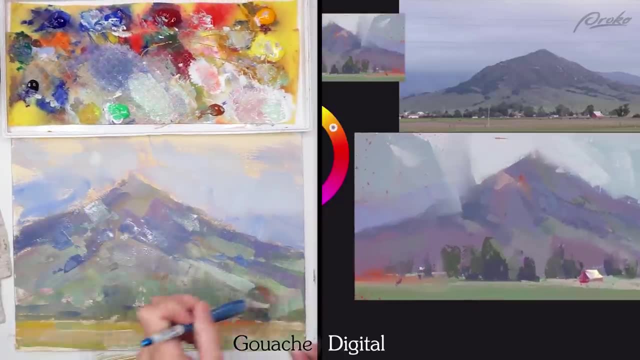 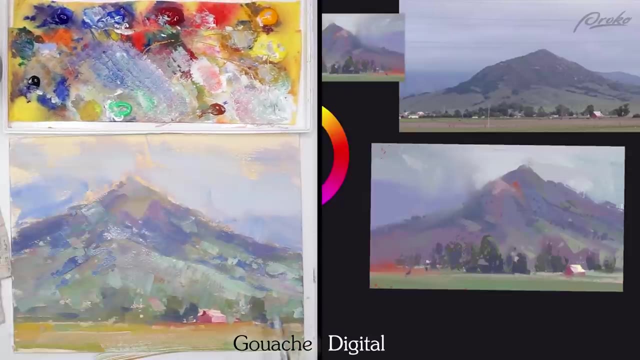 you just won't get the same results in colors. Nonetheless, painting traditionally helps you explore color relationships physically, right in front of you And, honestly, it can't get better than that, Once you slowly understand and unlock the attributes of color, such as value, color temperature and saturation.